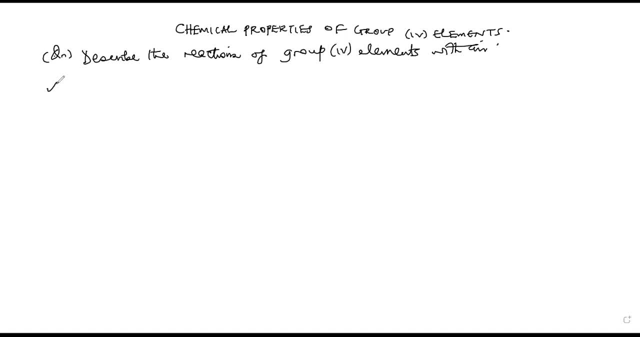 okay, uh, now the component of air that is going to be involved here is particularly oxygen, not any other. so one can say: reaction with uh described reactions of oh no as one. when i one one is answering one can say maybe certain element reacts with oxygen as a component of air. 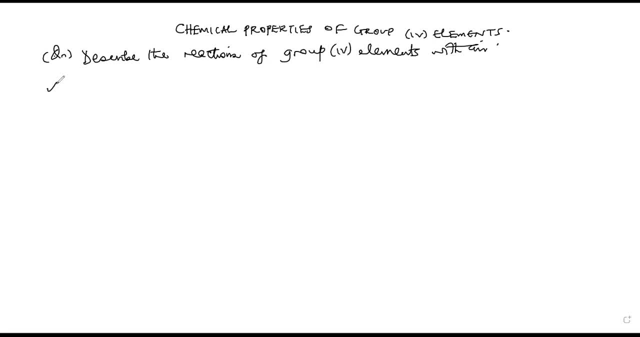 or since the only component of a involuntary can say reacts with air. right, so let's begin my answers. when you're describing the reactions, you have to give me the condition- your description must have conditions of reactions, the products and the equation. so, for example, with the carbon, 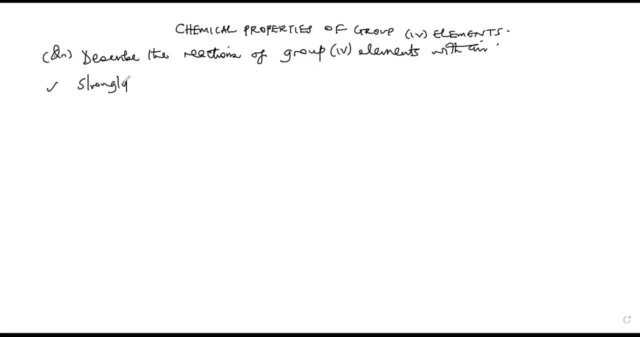 that carbon must be strongly strongly heated. strongly heated carbon reacts with air to form carbon dioxide, so we shall have carbon plus oxygen. oxygen from carbon dioxide, strongly heated, works with that form carbon dioxide. okay, then still for silicon. it will be strongly heated silicon. strongly heated silicon reacts with air. 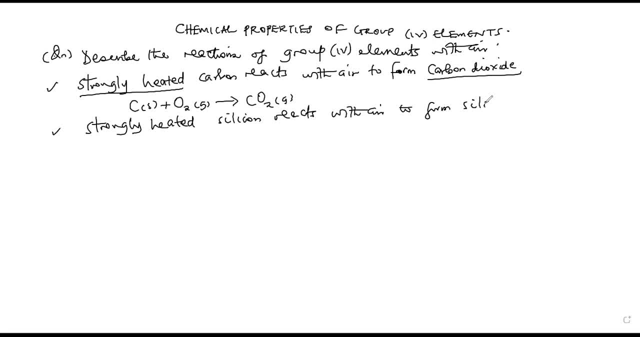 so we shall have silicon. so we shall have silicon plus oxygen. forming silicon dioxide is a solid uh-huh. then still strongly heated germanium. then still strongly heated germanium Reacts with air to form germanium oxide. You write the equation: germanium plus oxygen will form. 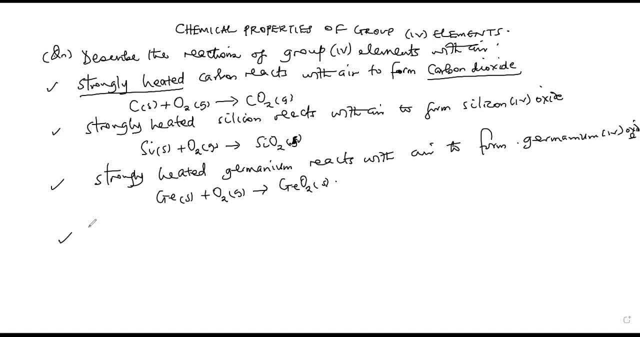 germanium oxide. Then we've got strongly heated tin Reacts with air to form tin oxide. So we shall have tin plus oxygen will form tin for oxide. okay Then with lead, heated lead it burns in air, But for it it forms lead two oxide, not lead four. 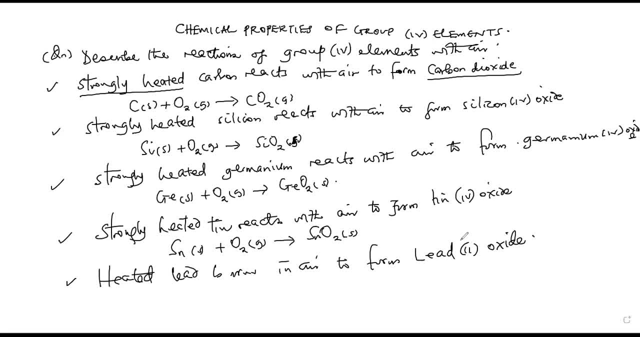 Because the lead in the plus four oxidation state is unstable, meaning it can undergo decomposition. Okay, When we form lead four oxide, it will undergo decomposition. so we form lead two oxide, which is stable. The final compound should be stable. So that is where the oxidation state idea has come about. 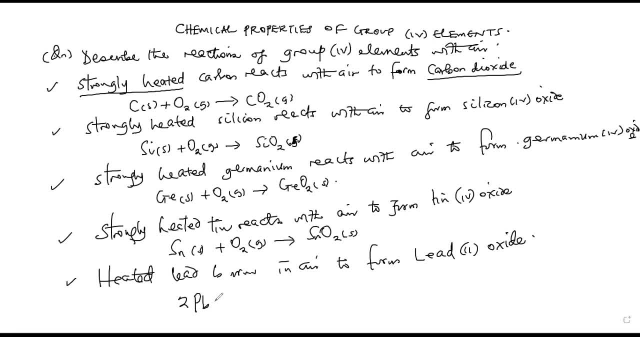 So we shall have lead plus oxygen will form two lead, two oxide molecules. You must form a stable compound. So this is how these react with the. this is how these compounds, this is how we do it. Okay, Okay, Okay, Okay. 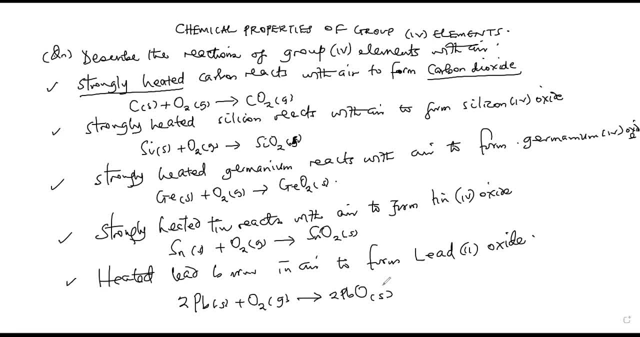 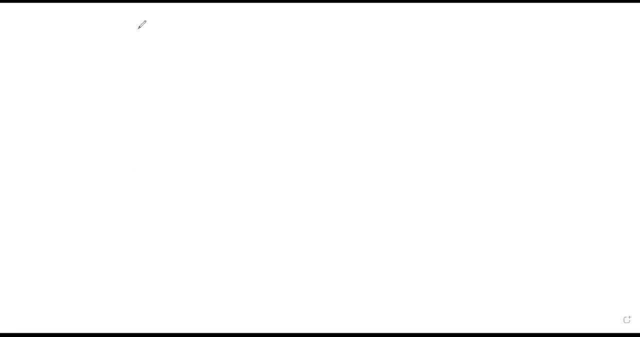 Okay, Let's take a look at how these elements react with the air. Let's look what reactions with water Reactions with the water. How do these elements react with water? Carbon, silicon and germanium and tin. they don't react with water. 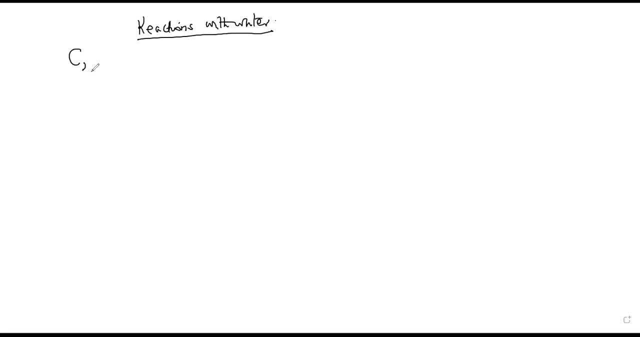 If the question is describe the reactions, then you have to tell me that carbon, silicon, germanium, tin do not react with water. Actually, let's say with the cold water. They don't react with cold water, but we have seen that they don't react with cold water. 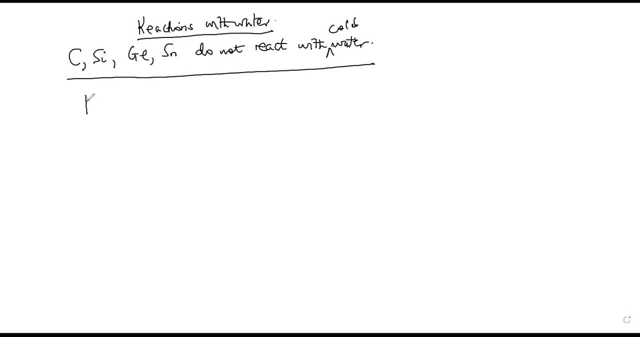 But if it is red hot carbon, red hot carbon- I'll first mark this because you've told me the conditions under what. they don't react with water, So that is, they don't react. They don't react with cold water, but red hot carbon slowly reacts with the steam and this reaction is reversible. 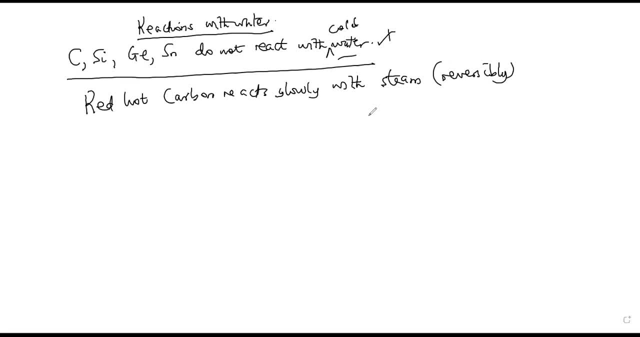 So reversible- react with the steam to form carbon monoxide Monoxide and hydrogen gas. The mixture of these two gases is actually called a water gas. So when carbon reacts with the steam, Steam is what a gas has formed. We form carbon monoxide- reversible. 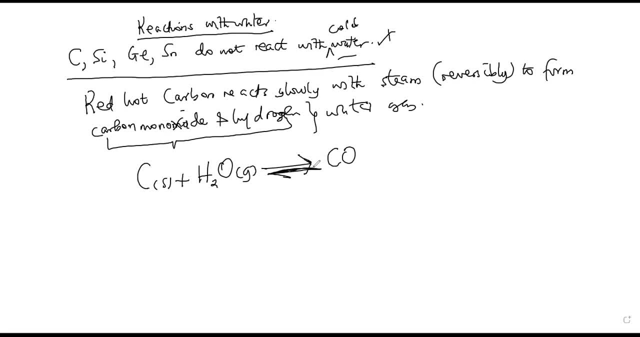 from carbon monoxide gas and hydrogen gas. you have to be specific with which carbon and which type of water that's reversibly with the steam from carbon monoxide. i told you that conditions can need to be marked and the products and the equation on a good 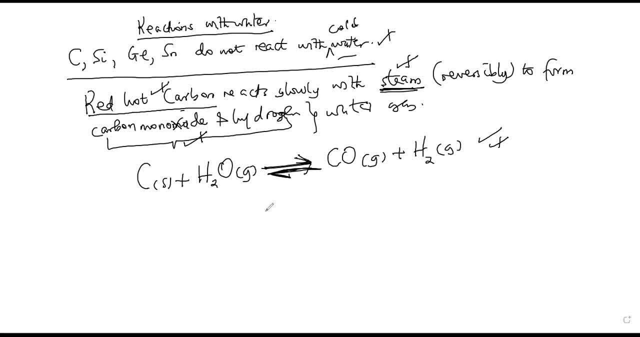 day, or one mark, one equation. then ready: hot silicon, red hot silicon reacts with steam to form silicon for oxide and hydrogen gas. so we shall have silicon plus steam, giving us silicon dioxide or silicon for oxide solid, then plus, of course, hydrogen gas. germanium, at any condition, does not react. 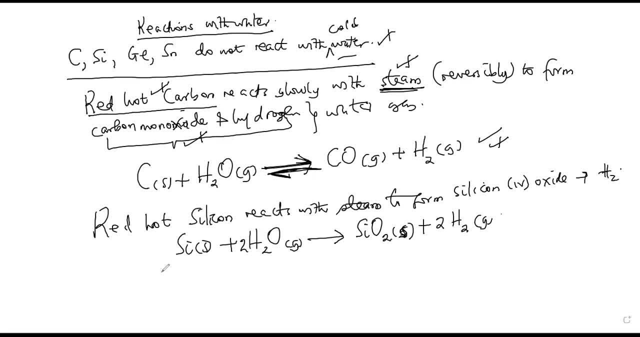 the water. but ready, what tin? that's with the steam from 24 oxide and hydrogen. so it will be tin plus steam to form 24 oxide plus hydrogen gas. these numbers of inorganic chemistry, you can really understand them by practice, the more you practice the things. 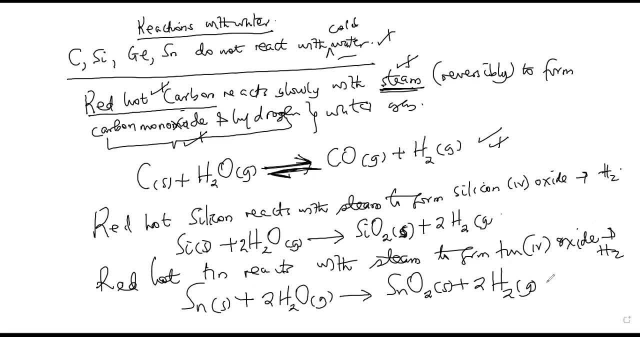 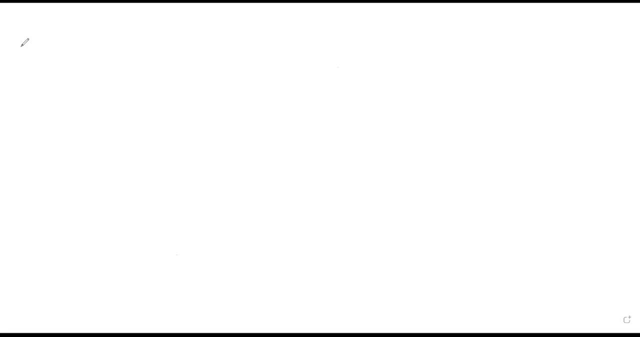 the more easy they become. okay, the more you practice them, the more easy they they become, because here it's a matter of knowing under what conditions. i'm going to do a summary at the end, then, for lead. lead must react with the only soft water containing dissolved oxygen. okay, so lead for it. 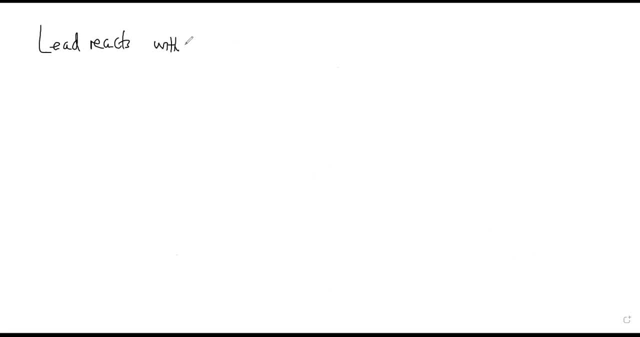 it reacts with the soft water which contains dissolved oxygen, and we form a solid product of red dried oxide. you have lead plus water containing resolved oxygen from lead to hydroxide. this is how we do it. now we found out that for reactions with water, of course, we've got carbon, we've got silicon, we've got. that is, in summary, onderling the 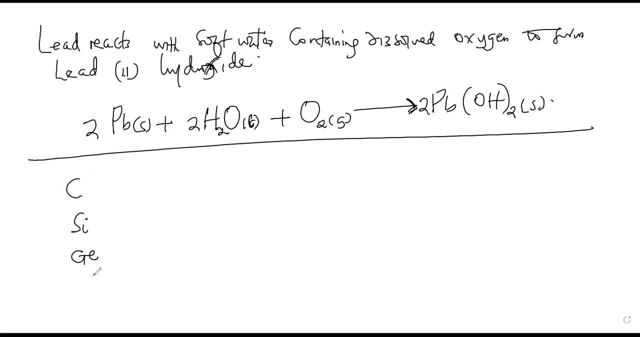 summary: we've got silicon with germanium, we've got tin and lead, carbon. it just cabin doesn't mean going. yeah, we are nicely rich, yeah, we are well rich, you can get new water, but which is the video? the video of my life? we are enter hemosaris tam TJ. we are getting invest in an alcohol. 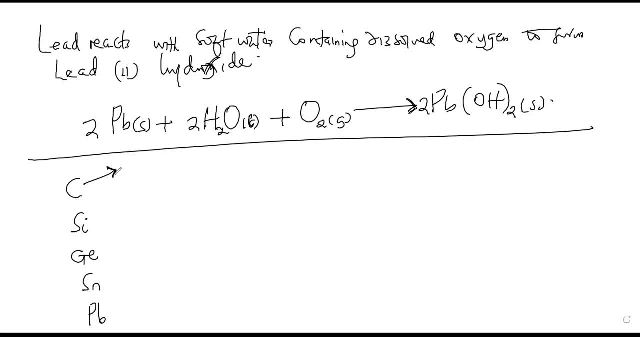 he gets a lot for this tool, Similar. no, you plant. contact us your brand. we get fat. you know now at least здism. carbon doesn't react with water, but ready-hot carbon reacts with steam to form carbon monoxide and the reaction is reversible. 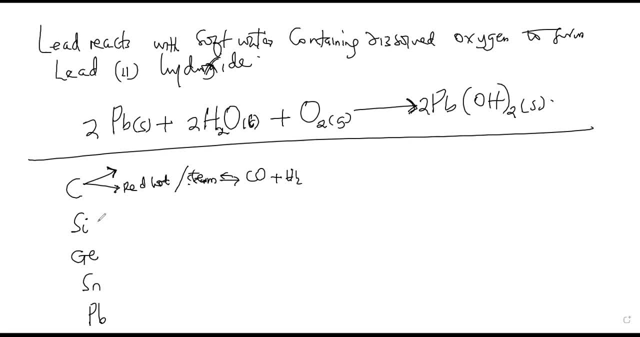 So we form carbon monoxide and hydrogen This silicon. it must be ready-hot And it also reacts with steam. That is how you get them. Germanium does not. at any condition. Tin must be ready-hot. OK, Tin must be ready-hot. 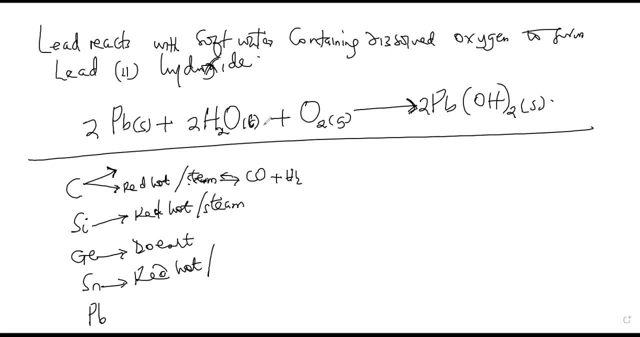 And reacts with it- Tin must be ready-hot- And reacts with it With the steam to lead. just reacts with the soft water containing dissolved oxygen. So you need to know under what conditions and what products do I form. So that is the reactions with water. 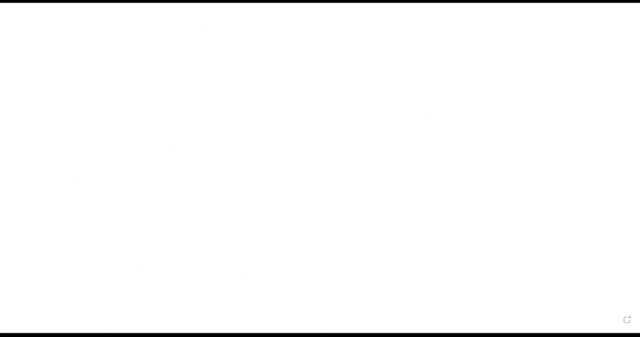 Then from there, OK, They can tell you to describe now with dilute acetazane, conservative acetazane. describe how group 4 elements and then group 5 elements and then group 6 elements and then group 7 elements and then group 8 elements and then group 9 elements and then group 10 elements. 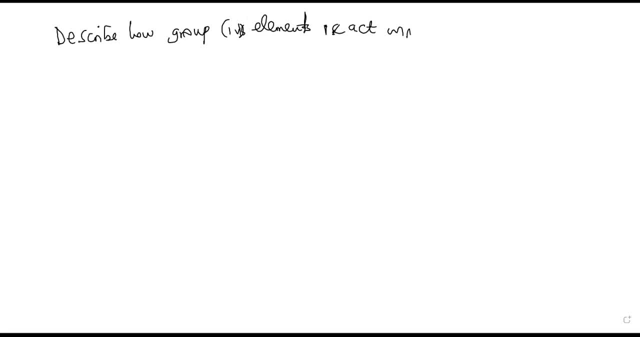 So the second one, I'm saying group 10 elements and then group 9 elements. Next, how does the human left react with, Reacts with? How does it react? How does it react with? How do they react with? 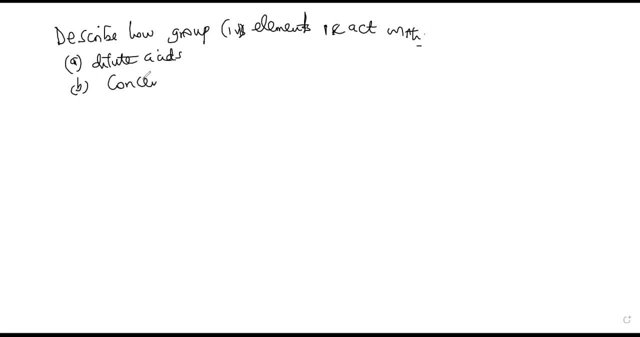 Reacts with One. That is, acids to concentrated acids, That is, acids to concentrated acids. Now Now in with dilute acids. When we talk about dilute acids, we've got a series of these dilute acids. We've got dilute hydrochloric acid. 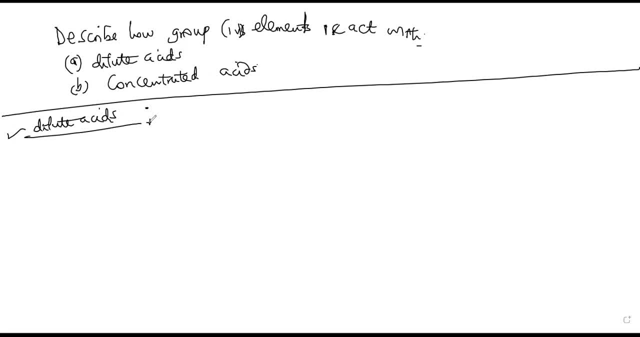 we've got sulfuric acid, we've got nitric acids. So when you look at dilute acids, if we are to begin with the hydrochloric acid, with the dilute hydrochloric acid, it first note for me that carbon is a very important 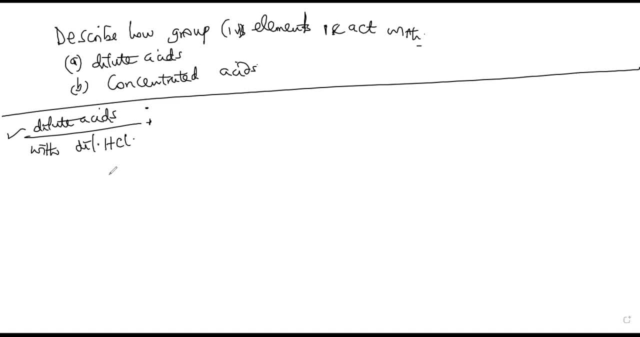 component of the process of diluting acid. It's a very important component of the process of diluting silicon. silicon, germanium- These ones, they do not react with the dilute hydrochloric acid. okay, They do not react with the dilute hydrochloric acid. 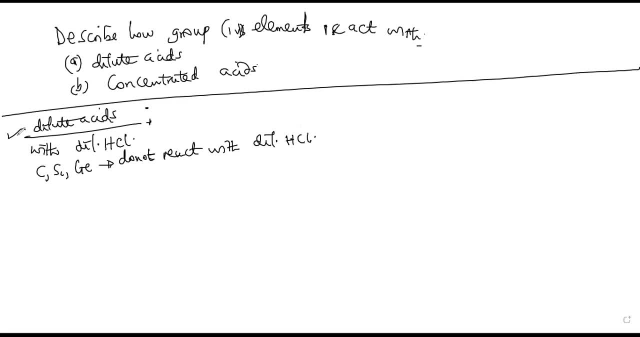 But tin now, tin is a very important component and now it means that tin and lead do. but let's see, Tin reacts with cold, dilute hydrochloric acid to form tin chloride and hydrogen gas. You have seen that tin that's with the hydrochloric acid. 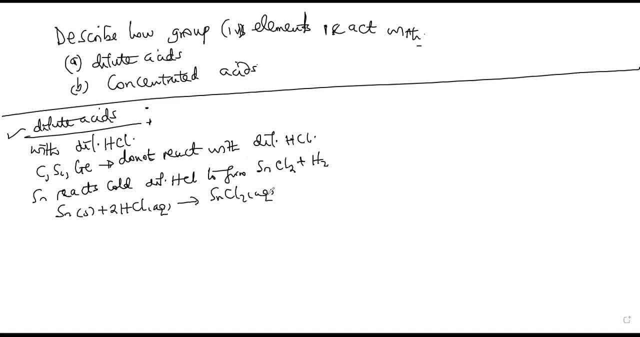 to form tin chloride and the hydrogen gas. All right, Lead. now there is lead. Lead reacts, but slowly because you formulate to chloride, which is lead, Which is insoluble, and the reaction soon stops. So lead reacts slowly with the dilute hydrochloric acid. 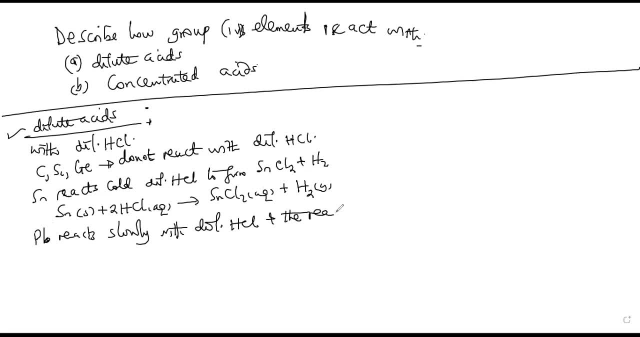 and the reaction stops due to formation of, formation of of insoluble. formation of insoluble lead to chloride. Formation of insoluble lead to chloride. Since the reaction soon stops, or since the reaction stops, we do not need to write the. 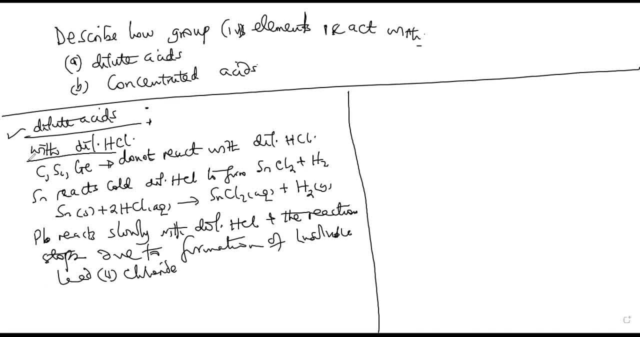 reaction there. So that is with dilute hydrochloric acid, Then with the dilute sulphuric acid, With dilute sulphuric acid. for dilute sulphuric acid we need to note that steel, carbon, silicon, germanium, these ones- Carbon, silicon, germanium. they do not react with dilute sulphuric acid. Even tin- carbon, silicon, germanium, tin- do not react with the dilute sulphuric acid, But lead, Lead, Lead Lead. 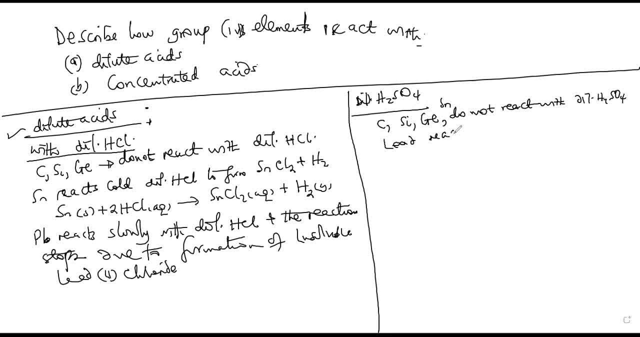 Lead. Lead Slowly reacts with it, So it reacts with dilute sulfuric acid and the reaction stops The formation of insoluble ED2 sulfate or insoluble ED2 sulfate. that is it. That is what I can talk about: dilute sulfuric acid. Let's look at dilute nitric acid. With dilute nitric acid you need to first note that carbon, silicon, germanium do not react with dilute nitric acid. do not react with dilute nitric acid, But for lead and tin they do. 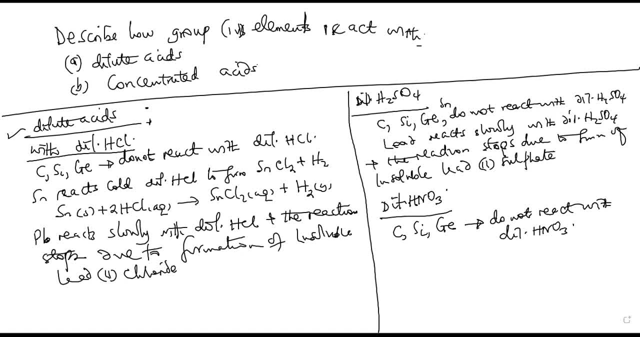 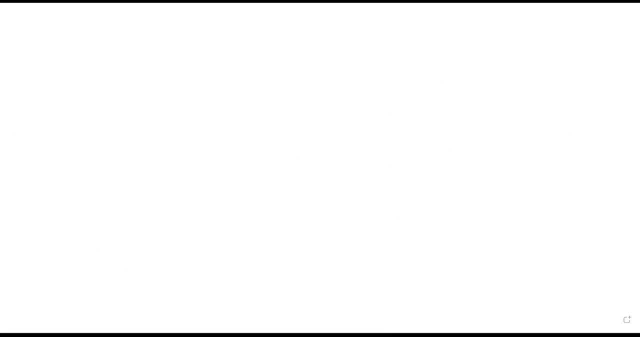 We are going to see how. So it would mean that when the acid is called dilute- because now, if the other three do not react, it means tin and lead do. so let's talk about tin and lead called dilute nitric. 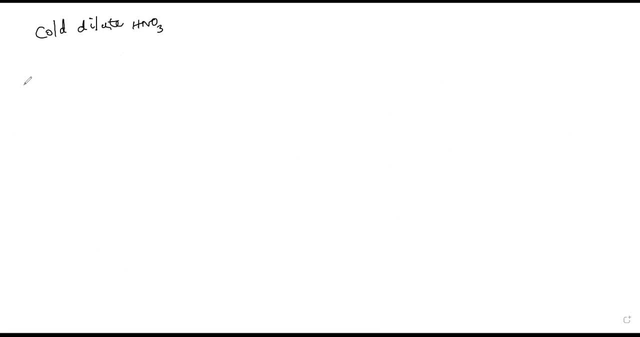 acid. If these twonote hate with want him to liked with Mitahaha, Can we add tin and lead Noroex, or at least be chosen? Mincred activate in the form of JMこみ İО Stitches Reduces tin toื่ет through nitrate. 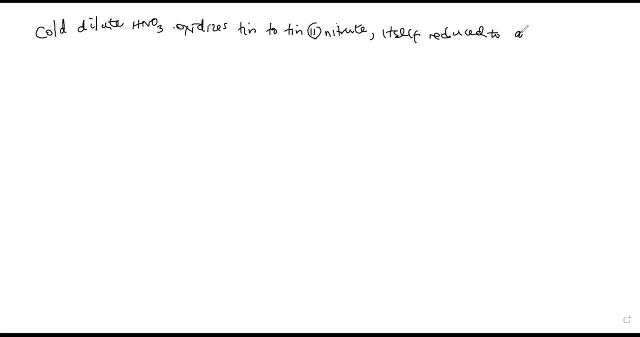 To respectively: Mincred occurs with lead perceptions. Itploat RIghtness, Divide nitrate and water. there's some stubborn reaction which is also undergone by iron and zinc. So we have said that tin reacts with coal dilute nitric acid. 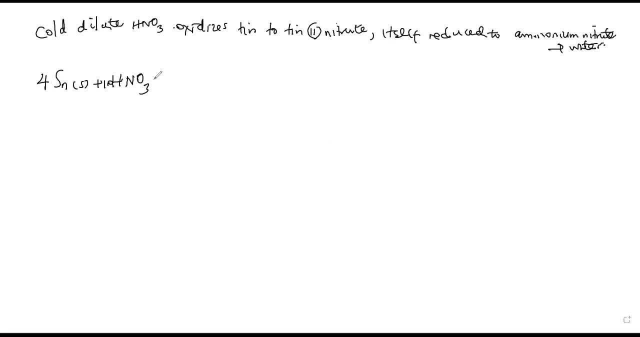 Tin molecules perform tin to nitrate and itself gets reduced to ammonium nitrate and water. So one can write still an ionic equation. One can write an ionic equation And this ionic equation is the tin plus hydrogen ions, forming two ions. 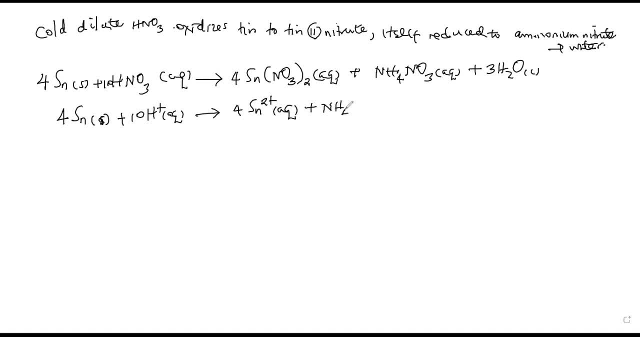 You have to write this equation very well: balanced, plus ammonium ion, plus the nitrate that comes with this nitrate, Then of course this is the ionic equation. So this is the ionic equation. So this is the ionic equation. 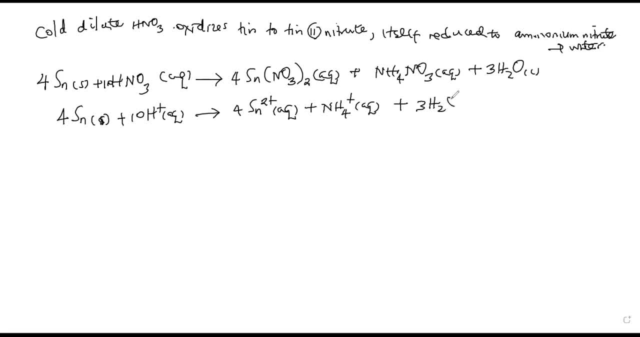 It's the ions plus the molecules of water. That is how it reacts. Then, for the case of lead, for lead to react, it has to react with dilute Or modulately concentrated Or half concentrated nitric acid. okay, so this one, this acid oxidizes lead. 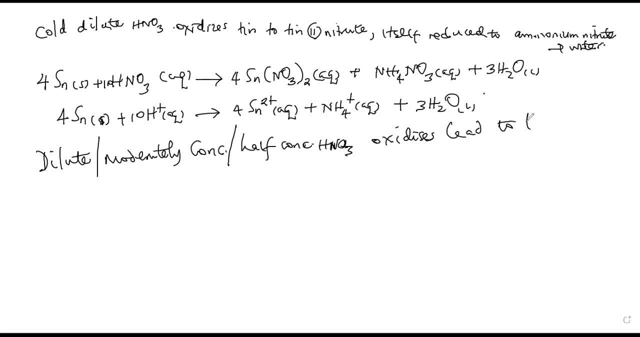 to lead to nitrate and itself is oxidized, is reduced, itself reduced to nitrogen monoxide and water. so we have said that lead, we shall have three lead atoms plus nitric acid. we form lead to nitrate plus nitrogen monoxide and water. ionic equation. you can write lead: 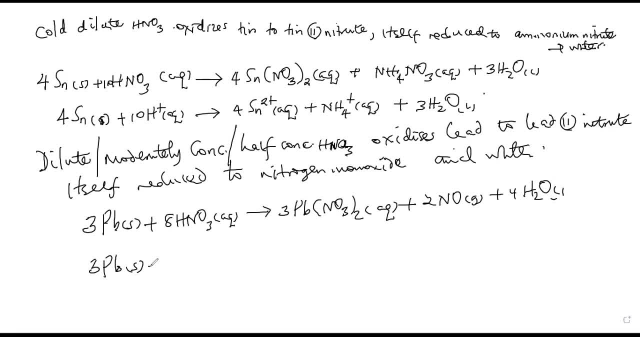 plus nitrogen ions, yeah, plus nitrate ions, will form. these are two nitrate ions, uh, three lead. these are supposed to be eight hydrogen ions, two nitrate ions. so from three, two ions, nitrogen monoxide and water. that is what we form, because in an ionic equation, gases and liquids do not ionize. 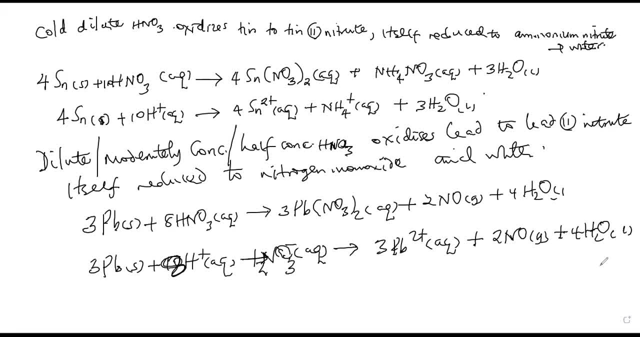 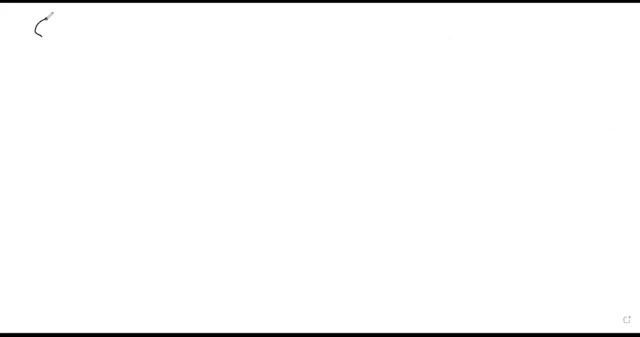 so, before we go to uh, concentrated acids, uh, there are some other acids with which these elements react, for example, silicon. silicon is the only element that reacts with the hydrofluoric acid. reacts with the hydrofluoric acid and when it does so, we form hexafluorosilic. 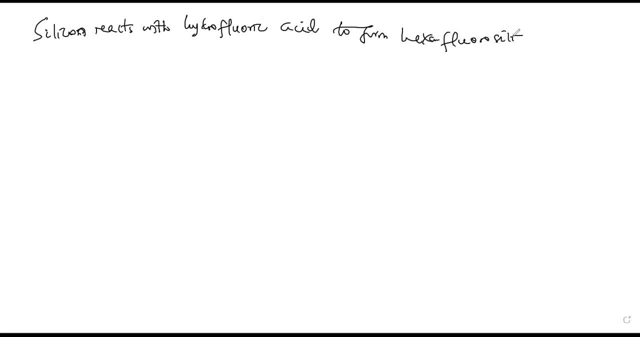 hexafluorol sillic acid, hexafluorosilic acid and hydrogen. so we're having silicon solid plus hydrogen fluoride. sorry, hydrofluoric acid will form hexafluoro silicic, hexafluoro hexa, meaning the fluorine atom is supposed to be six. 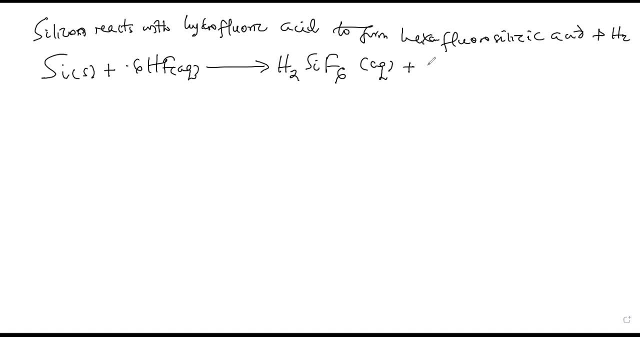 hexafluorosilic acid. that's it and hydrogen gas. also. lead can react with the ethanoic acid. these are reactions with other acids. lead reacts with lead reacts with the ethanoic acid and that reaction takes place in presence of air, in presence of oxygen or air. 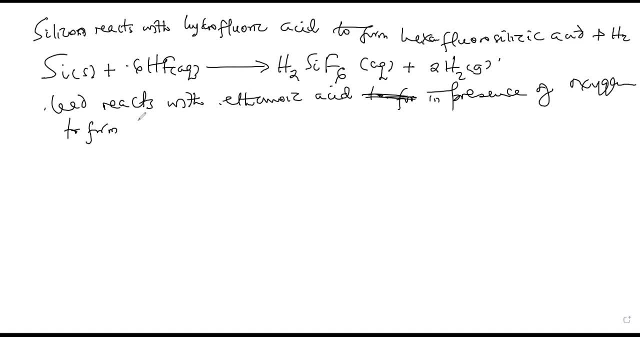 to form, lead to ethanoic and water. so we have lead to ethanoic plus ethanoic acid in terms of oxygen form, lead to ethanoate and water, so from there we can go to concentrated acids. so you should make your own summary and you see. 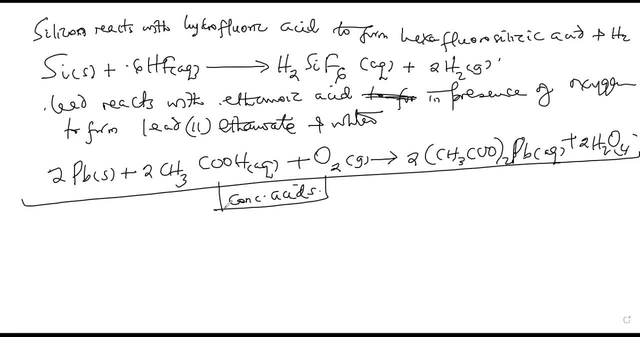 how they do. concentrated acids react with the variety of them and let's see how these reactions are with concentrated acids, of course, uh, concentrated acids we are also going to look at first with the conch hydrochloric acid, with conch hydrochloric acid, if you begin with hydrochloric acid. 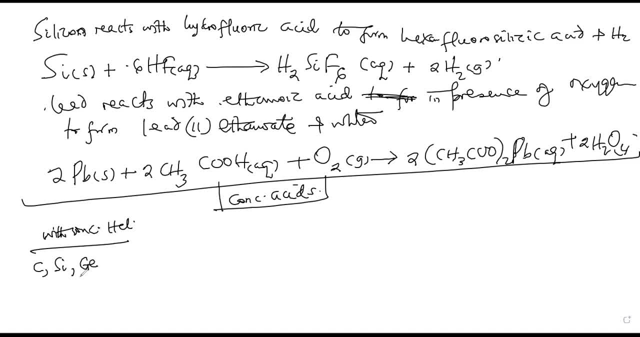 carbon, silicon, germanium, do not react with the conch hydrochloric acid. these ones, they do not react with the conch hydrochloric acid. but tin reacts vigorously. when you're writing for us, don't write acid. writing reacts vigorously with the hot conch hydrochloric acid. 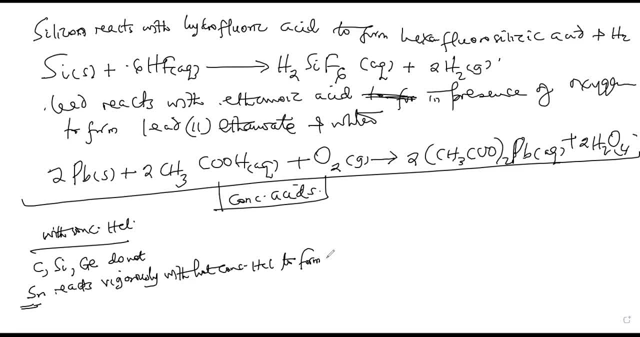 from tin to chloride and hydrogen to form tin to chloride and hydrogen. so we shall obtain連 solid plus. lead can react with the boiling hydrochloric acid. boiling constituted hydrochloric acid, it form lead to chlorideочки. also lead can react to with the boiling hydrochloric acid, boiling concentrated hydrochloric acid, causing a. 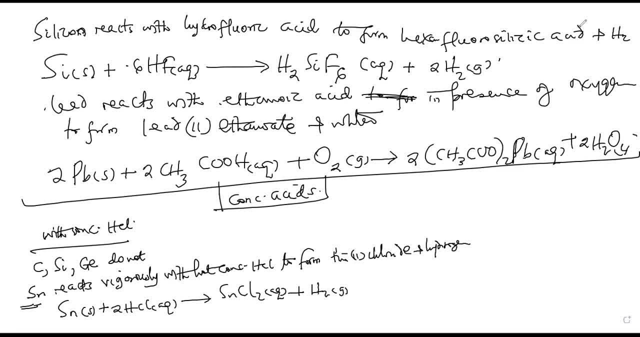 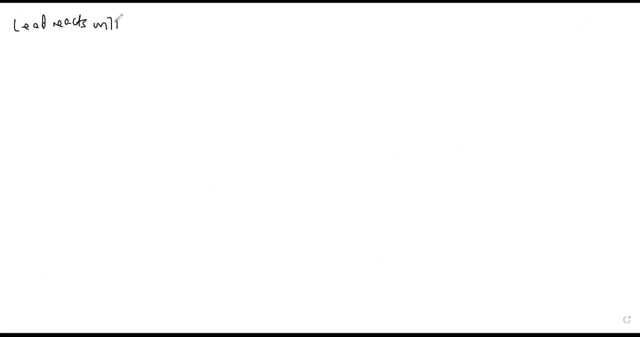 chloride and hydrogen. okay, so also now. lead reacts with the boiling conch hydrochloric acid to form lead to chloride and hydrogen. so looking at that, it is lead solid plus boiling conch hydrochloric acid appears form lead to chloride and hydrogen gas. that was the concentrated 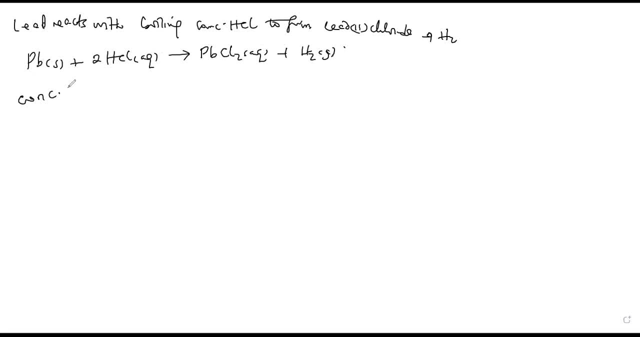 hydrochloric acid. two, when we look at concentrated sulfuric acid, this one is a strong oxidizing agent and most of its reactions are going to be with uh. most of its reactions are going to be with the compounds which it uh, with the compounds that it does what that it oxidizes, for example, 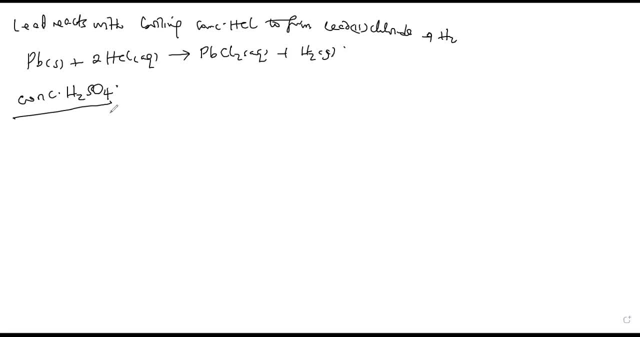 uh, for example, we are going to say that: uh, yeah, let's begin with the carbon hot conch. sulfuric acid oxidizes carbon, carbon dioxide, and it's soft, reduced to sulfur dioxide, water when you're writing these words, that's sulfur dioxide, those are two words, and water. so equation: we have carbon solid plus. 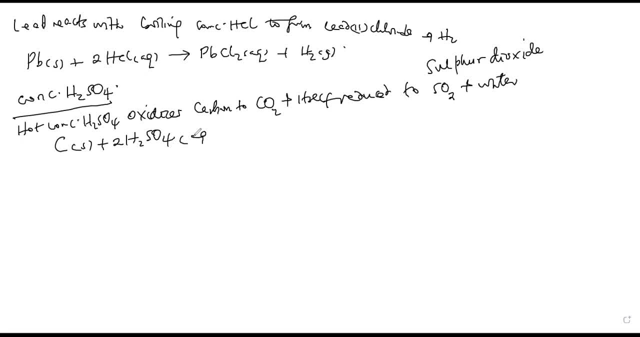 conch rich acid, we shall form carbon dioxide gas and it's sort of various sulfur dioxide gas and water liquid, uh, silicon- that was carbon silicon and germanium. they do not react with concentrated sulfuric acid, but tin is oxidized, so hot coke. sulfuric acid, being an oxidizing agent, oxidizes. 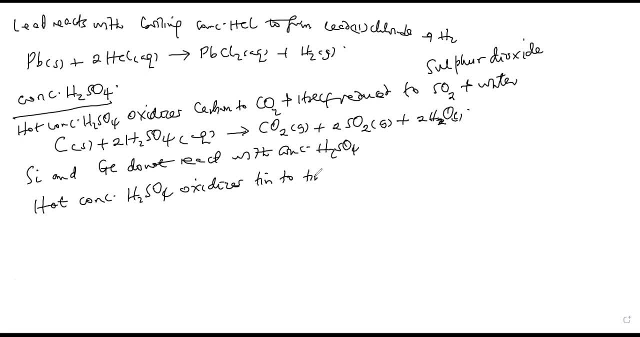 tin to tin for sulfurate. tin for sulfurate and itself reduced to sulfur dioxide and water. sulfur dioxide and water. what does it mean? we have tin solid. it is oxidized by sulfuric acid and we say that we found tin for sulfurate. if you think for sulfurate, mean that the variance of tin is fun. the surface is too so. 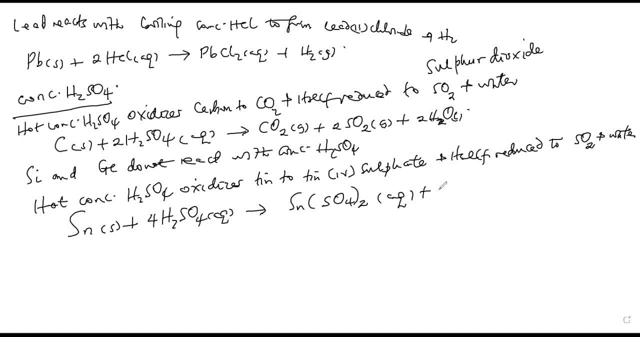 shall have tin for sulfate, as this and itself is reduced to sulfur dioxide and water, because we need to know the aspect of oxidizing agents and reducing agents and oxidizing agent is reduced. so, since sulfuric acid is an oxidizing agent, at the end of the reaction it is reduced to turhedium backs on water. 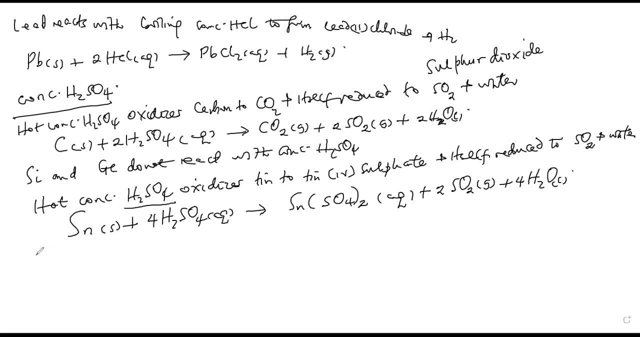 so that is thin. then lead concentrated- you have to write the whole word Forty: concentrated sulfuric acid oxidizes lead to lead to sulfuric and self-reduced to sulfur dioxide and water. So we shall have lead plus sulfuric acid, shall form lead to sulfuric and so forth be reduced. 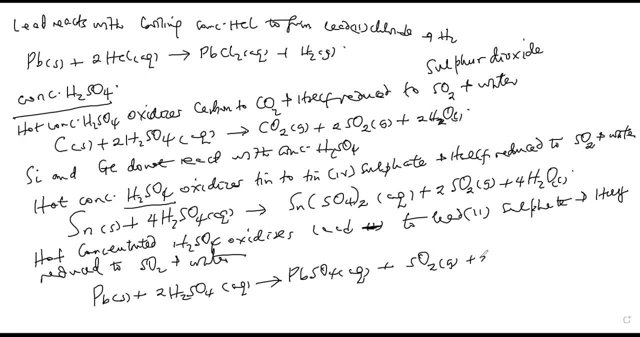 to sulfur dioxide and water. The best thing here is to learn how to balance these equations, and they stick you to your head Now. it means that for this reaction with sulfuric acid, it is carbon, tin and lead that undergo it. So when they said, describe the reaction with the, describe the reaction of the reactions. 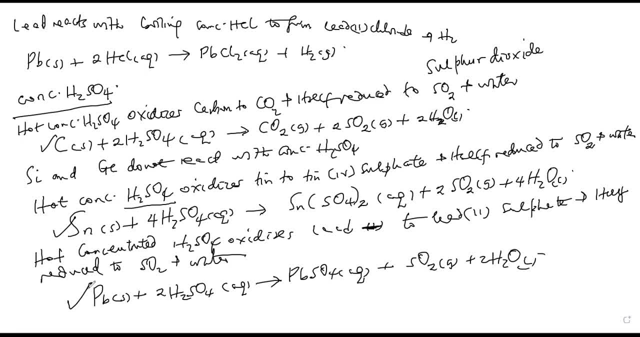 of group four: elements with dilute acids, talk about dilute acids with each element. If they say with the concentrated acids, talk about acid. But if they say Acid is just, You have to talk about dilute and concentrated and you have to give when. when the question. 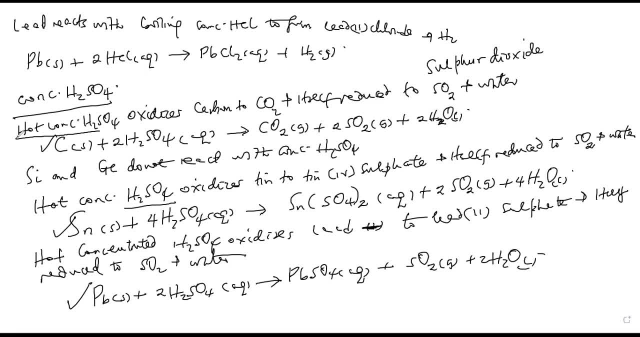 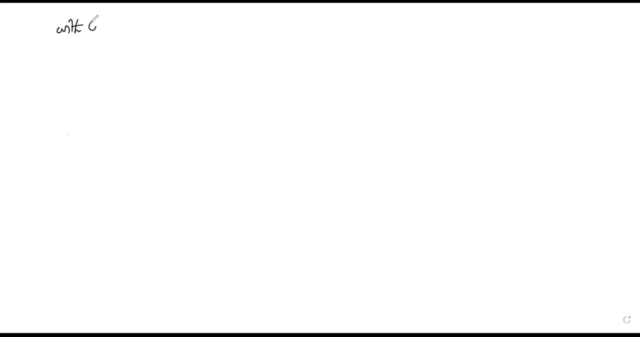 is just described. you have to give us the conditions in the reaction products formed and the equation. as simple as that. Let's go to conch nitric acid. Okay, With the conch nitric acid, With the conch nitric acid. 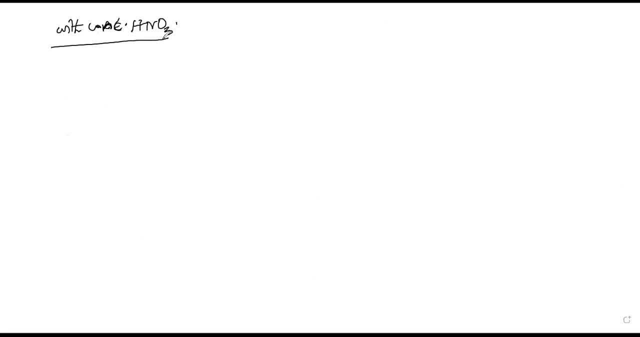 With the conch nitric acid. Okay, Um, Okay, Okay, Let's begin with the carbon Hot. It is also an oxidizing agent. Hot conch nitric acid oxidizes carbon to carbon dioxide. Those are two words. when you're writing words. 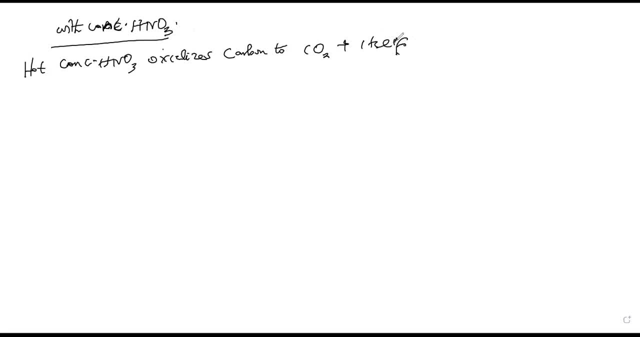 And so Reduced to nitrogen dioxide, nitrogen dioxide and water. I'm using formulas because of maybe time and the work we have to cover, But make sure you use words. So equation: we have carbon plus nitric acid, what you call nitric acid. 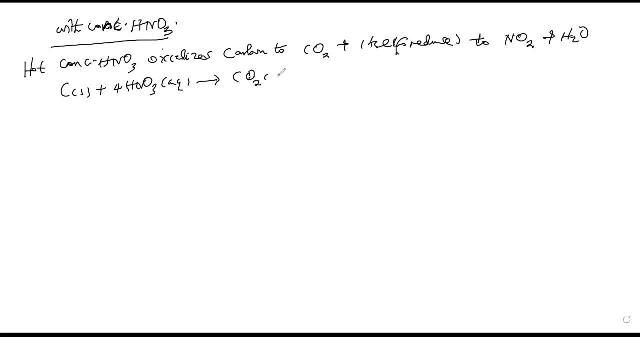 We say that it oxidizes carbon to carbon dioxide and itself gets reduced to nitrogen dioxide and water. Then silicon: now that is carbon. So silicon does not react with the conch nitric acid, But when we go to germanium hot conch nitric acid, it oxidizes germanium. 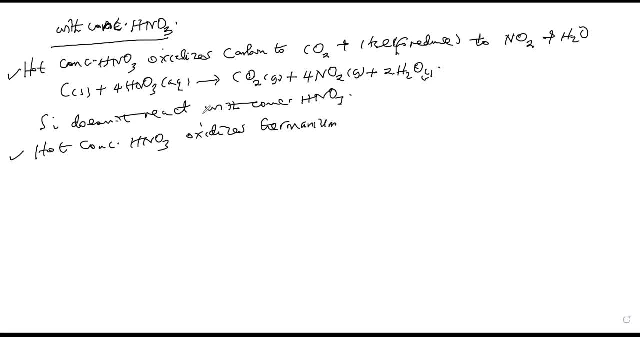 Or germanium to germanium for oxide. germanium for oxide Being an oxidizing agent, itself is reduced to nitrogen dioxide and water. Equation: germanium solid plus conch, nitric acid from germanium for oxide, and itself is reduced to nitrogen dioxide and water. 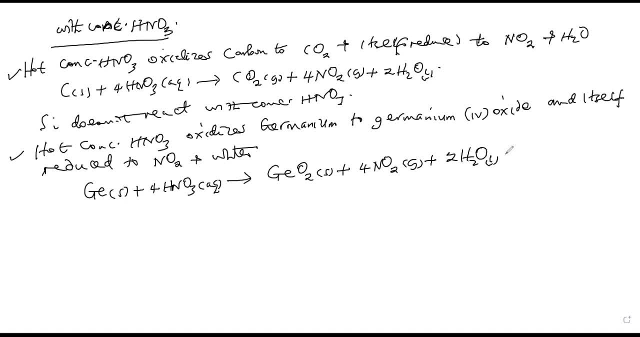 So it's a matter of knowing which one is reacting, Which ones do not react, Under what condition? it must be hot conch From what? germanium for oxide and nitrogen dioxide and water. Still hot conch. nitric acid. hot conch nitric acid oxidizes. 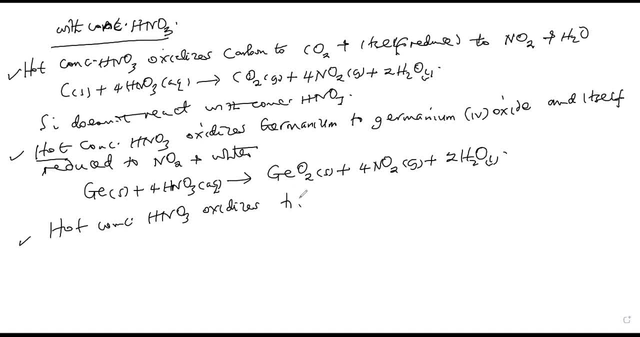 Tin. So there is a tin, Two tin for oxide And itself reduced to nitrogen dioxide and water. Okay, And that equation can be written: the same balancing scheme, So we have tin plus nitric acid, molecules from nitrogen dioxide and water. 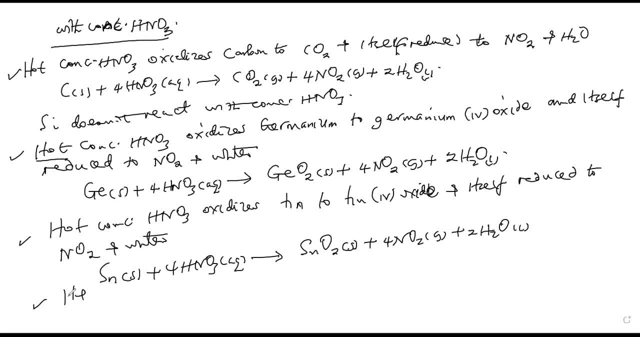 Lead, hot conch nitric acid. hot conch nitric acid oxidizes lead to nitrate and it's soft Reduced to two, nitrogen dioxide and water. How do we write this equation: Shelf lead plus nitric acid? 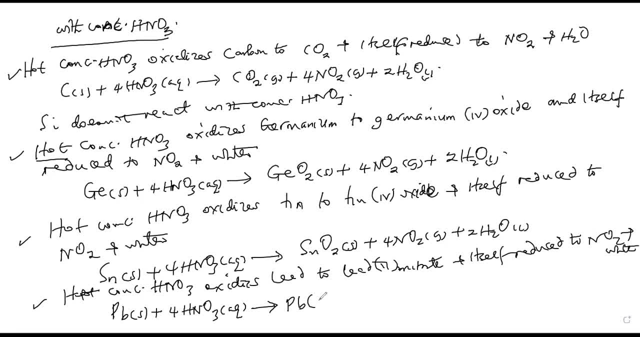 Shelf lead to nitrate and it's soft- would be reduced to two. You will fetch all your marks. Anything is easy to learn. It's a matter of knowing which one is reduced to what Those apart from lead, Others are oxidized to their dioxides. 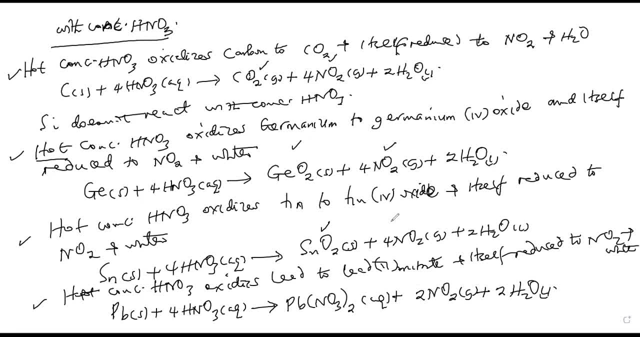 Throughout you form nitrogen dioxide gas and still throughout water. The balancing points on nitrogen dioxide gas are equal 4, 4, 4.. Water: 2, 2, 2.. Nitric acid: 4, 4, 4.. 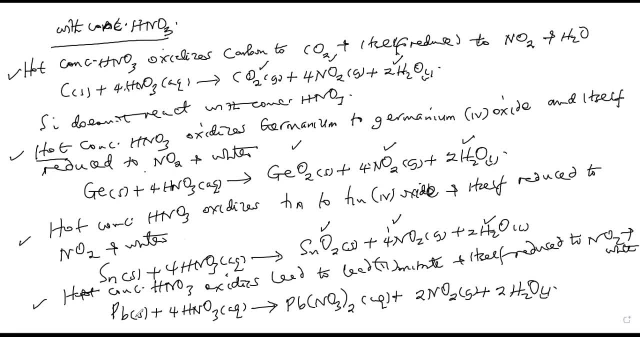 You see. So it's a matter of knowing 4, 4.. 2, 4, 4, 2.. Very simple, So it is always easy to get all the marks on an inorganic chemistry equation. Very, very, very easy. 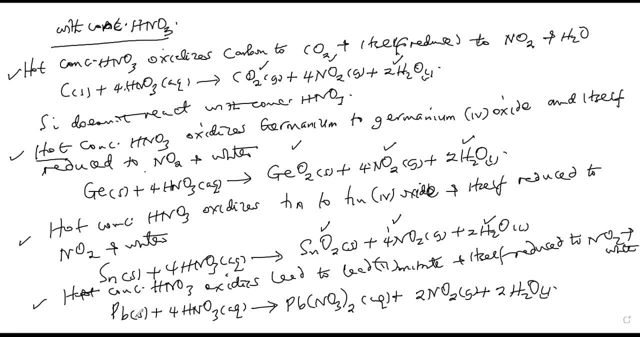 Quite easy, Quite easy to get all the marks, OK. So now those are the reactions with acids. Now with alkaids, because I want to record all the reactions of these elements in one video. So let's look at with alkaids. 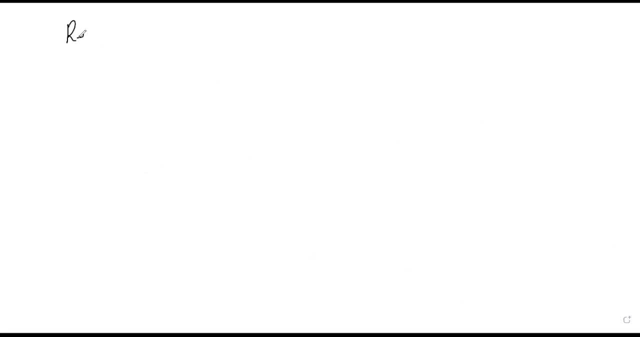 Reactions with dilute and concentrated sodium hydroxide. I've specified an alkali, but even if they say potassium hydroxide, they are the same. Let's begin with dilute. OK, OK, We dilute alkalis. 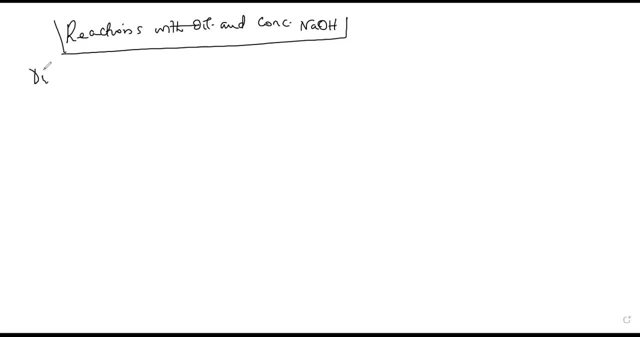 OK, We dilute sodium hydroxide. We dilute alkalis. OK, We dilute sodium hydroxide. I'll summarize this for you: Carbon does not react with either dilute or concentrated sodium hydroxide solution. So, to begin with, carbon does not react with either dilute or concentrated sodium hydroxide. 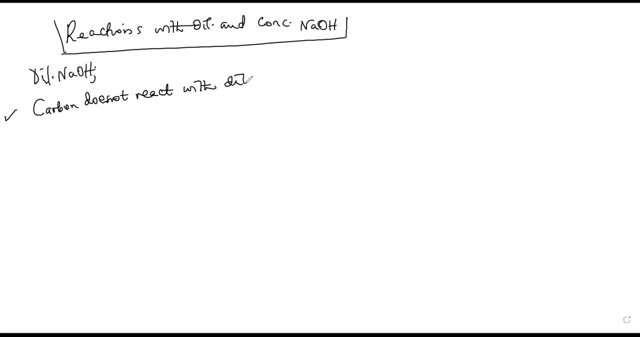 does not react with dilute and quarks sodium hydroxide solution. that is, carbon silicone reacts with both dilute and hot quark sodium hydroxide to form sodium silicate. from sodium silicate and hydrogen gas equation we have silicon solid plus sodium hydroxide solution. 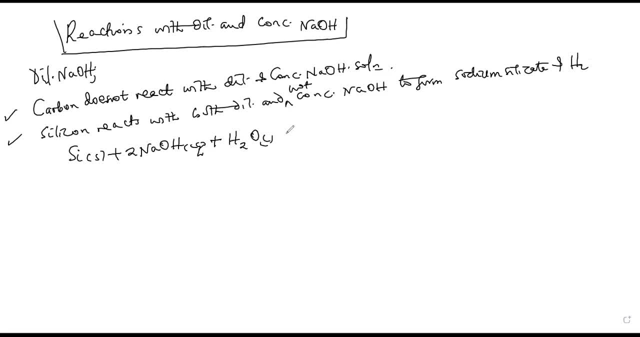 in presence of water, we form sodium, silicate and hydrogen gas. how do we write the equation? we have the ionic equation. you can say: all silicon plus sodium hydroxide plus water, you form a silicate ion and hydrogen gas. as simple as that. okay, then let me make it general. 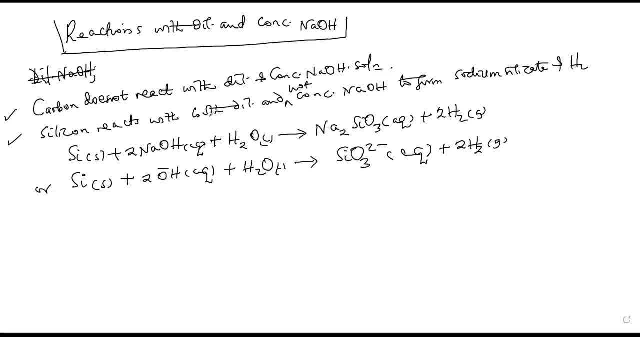 reactions with the dilute and cold. okay, so silicon is the one that reacts with both dilute and cold. carbon does not react with the dilute and quark. then germanium reacts with the hot quark sodium hydroxide to form. we form a sodium germic. 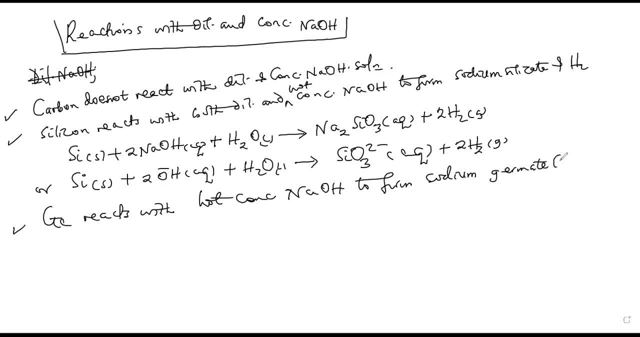 we form a sodium germic and hydrogen gas. with germanium we form a sodium germic four. but when it has reacted with 40 concentrated it does not react with quarry. how do you write the equation? you have germanium plus sodium, so Wide, So qua Plus. 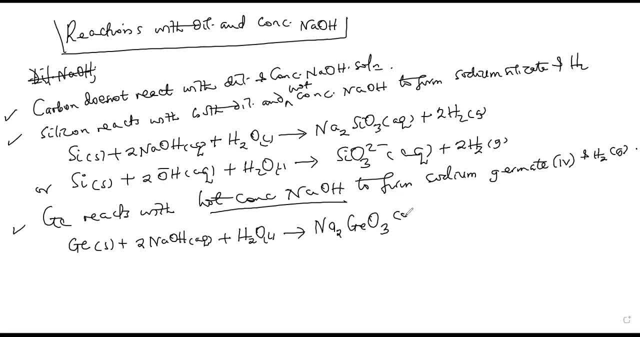 Hydroxyd Plus water You form so � reicht like this so diient mh4 sodium you have germanium solid plus hydroxide appears plus water we shall form sodium germate 4 plus hydrogen gas or or you can write germanium solid plus sodium hydroxide 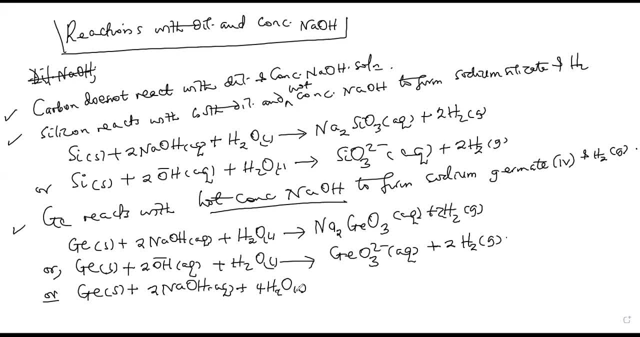 excess water. yeah, i've used four molecules of water and now still we've got four molecules of water. and now still we've got four molecules of water, and now still we've good form sodium, genette and hydrogen. you can write this ironically as germanium plus. 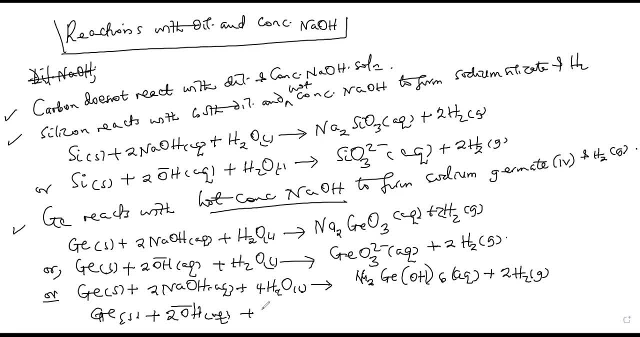 hydroxide ions plus photomolecules to form. now, for this case, we shall have a germate of us written as so. this is a germate ion, germate for iron aqueous and hydrogen gas. so out of these ones you can pick any equation and use it. 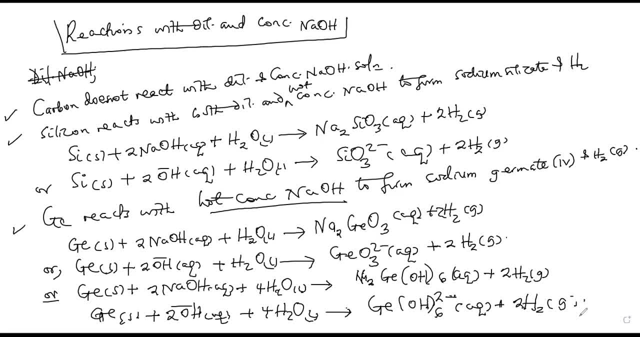 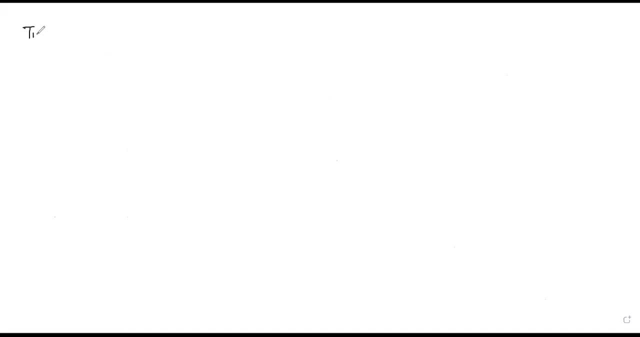 when it comes to the reactions of germanium, tin reacts the same way as germanium, but with the, also concentrated. okay. so tin reacts with the hot conch, sodium hydroxide, to form sodium stannate. for this we form sodium stannate four and hydrogen gas. i told you that one will mark what it reacts with under product. 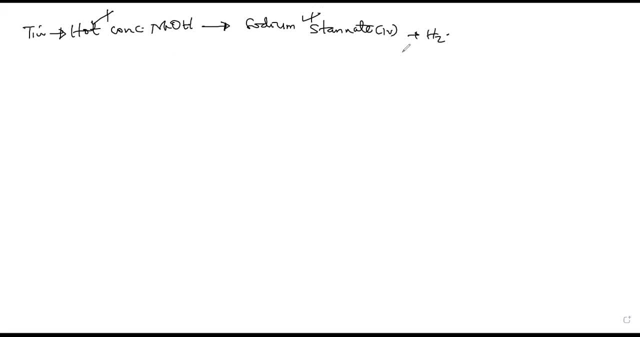 what consider sodium hydroxide from sodium stannate? four equations: you can write tin reacting with sodium hydroxide and water, uniform sodium stannate, perform and hydrogen. or you can write the ionic form of these plus two high dioxide iron plus water, you form SNO3, 2- and 2-hydrogen gas. 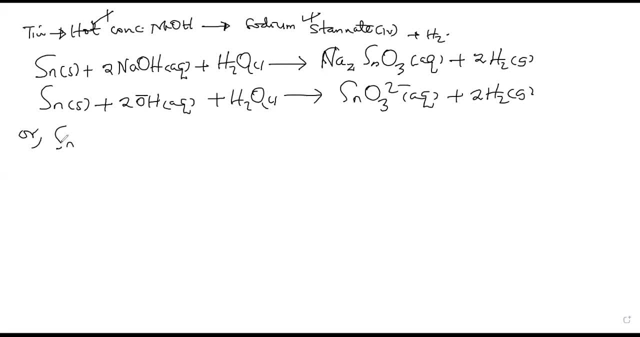 Or you can write tin plus sodium hydroxide plus four molecules of water, still you are going to form astanate. sorry, you are going to form N-H2, SN or H6 and hydrogen gas, Or still you can form. 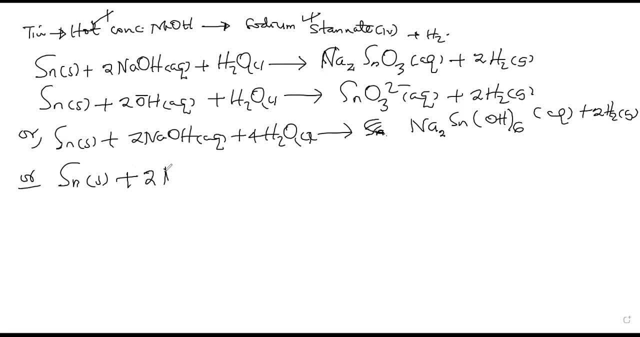 N-H2,, SN or H6 and hydrogen gas. Or still you can form SN or H6 with OH and four molecules of water. because water does not agonize, You form SN or H6, 2- and two molecules of hydrogen. 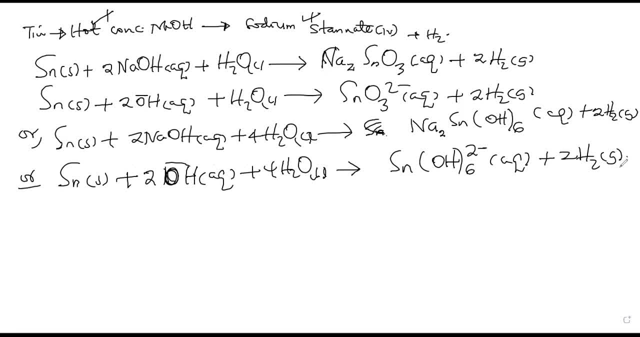 Any of those ones will earn you a mark. Now, that was tin With linge with lead. it reacts with hot, also hot conch. sodium hydroxide from sodium plambate from sodium plambate 2. sodium plambate 2. 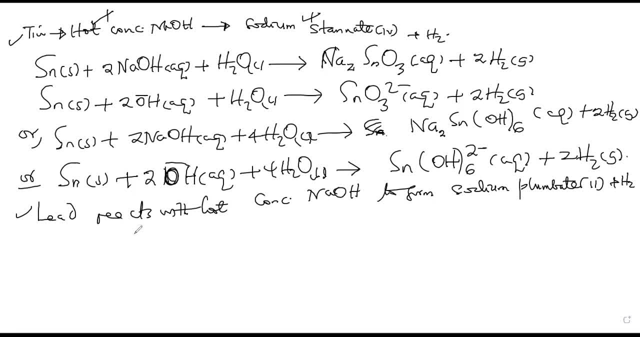 and automatically hydrogen gas equations. you can have lead solid plus 2 sodium hydroxide without water, you form a plambate- 2 and hydrogen. or you can have lead plus sodium hydroxide. sorry, sorry for this equation, sorry for this equation. let me repeat the first one. 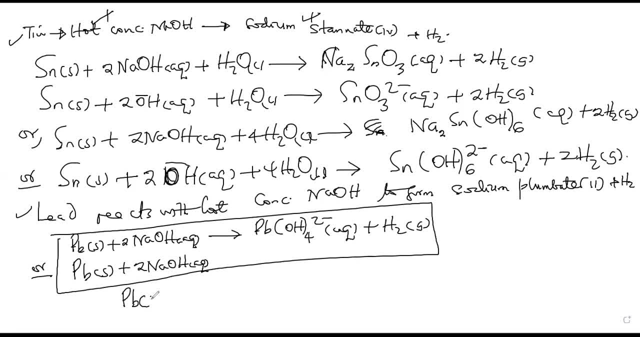 because it was supposed not to be ionic here. so lead plus sodium hydroxide, you form a plambate, sodium plambate 2. okay, yeah, yeah, yeah. sodium plambate 2 and hydrogen gas. or you can write the ionic form of this as: 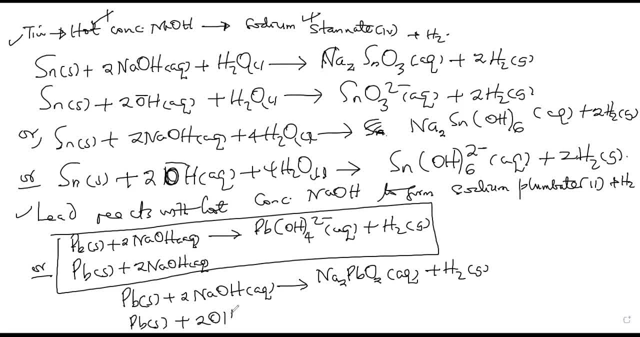 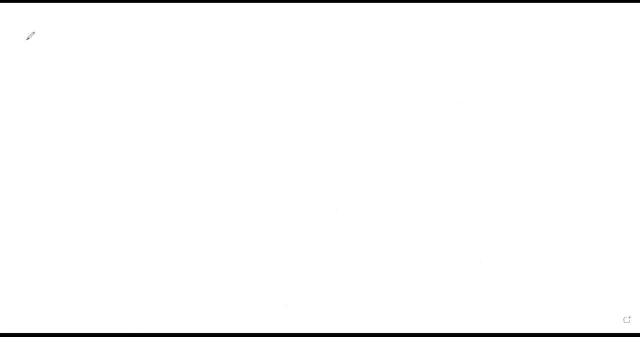 or you can write it when it's reacting with water in terms of water, so you'll have lead plus 2, sodium hydroxide plus water to form 2OH ions, to form sodium, plumb it and hydrogen gas, or lead plus 2OH plus water. 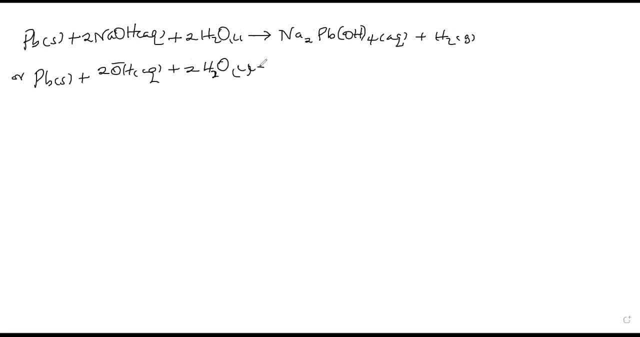 you form a plumbed pboh for minus two, minus rather plus hydrogen gas. so still, any of those, any of those can work. now we are left talking about. we are left to talking about the reactions with chlorine and then sulfur. okay, reactions of. with chlorine, they can tell to describe the reactions of group four, elements with chlorine, with chlorine of. 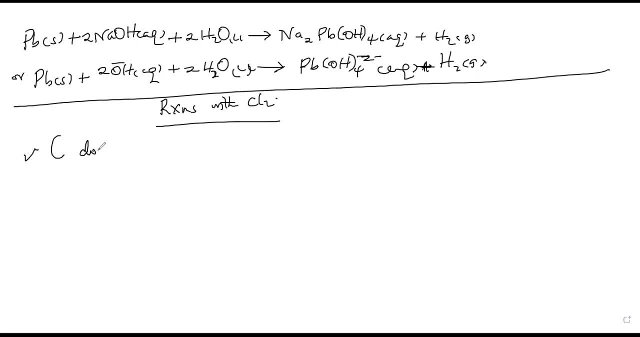 course you have to talk about. each carbon does not react with chlorine, ah two. the other ones have to react, but when they are heated, heated silicon reacts. with which kind of chlorine? dry chlorine, to form what? silicon tetrachloride form silicon tetrachloride. so we shall mark. 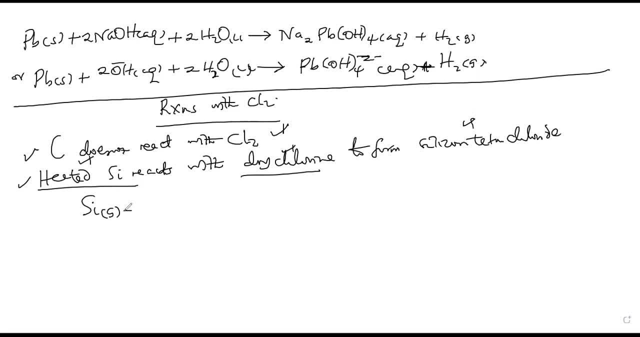 and then you write the equation silicon plus chlorine. how many two? we form silicon tetrachloride. this is a liquid, heated germanium reacts with the dry chlorine. from what? germanium 4 chloride? from germanium 4 chloride. you write the equation ge plus cl2. 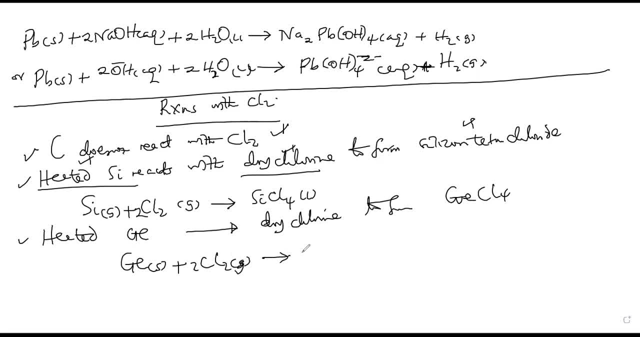 gas to form GECF4.. It's a liquid. Then we've got what we call heated tin. reacts with also dry chlorine to form tin 4 chloride. Yeah, yeah, yeah, Tin 4 chloride. I've tried that once, So we shall have. 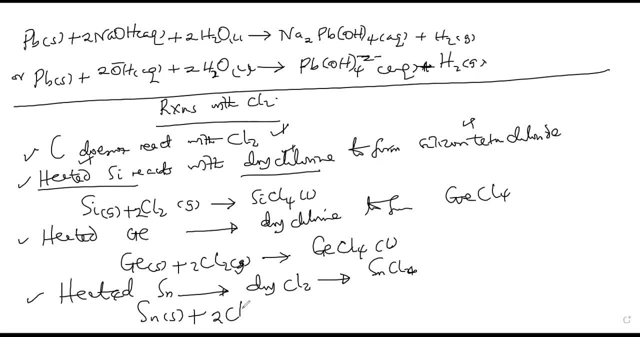 tin plus 2 chlorine molecules, You're forming tin 4 chloride Liquid. That is tin For lead. it must be also heated. Heated lead reacts with. when you're describing, you have to write words: Heated lead reacts with. 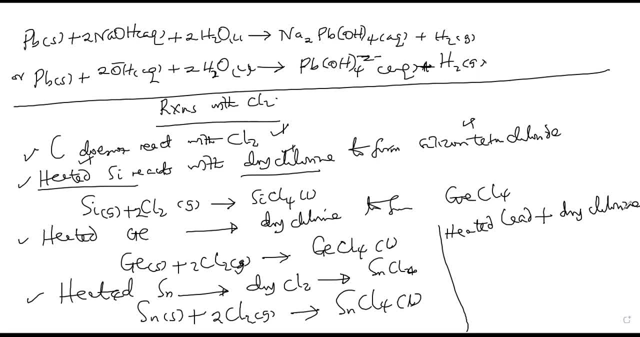 dry chlorine. Now for lead. we don't form lead 4 chloride, because lead 4 chloride is unstable. It will undergo decomposition. Instead, we shall form lead 2 chloride, And lead 2 chloride is not a liquid but a solid. 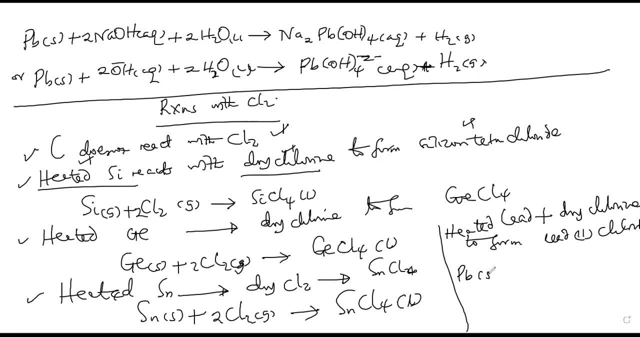 That is where students get it wrong. So for lead, it's a solid which reacts with chlorine gas to form lead 2.. So lead 2 chloride. You've known why we are forming the chlorides of the positive oxidation state. And for lead, we are forming 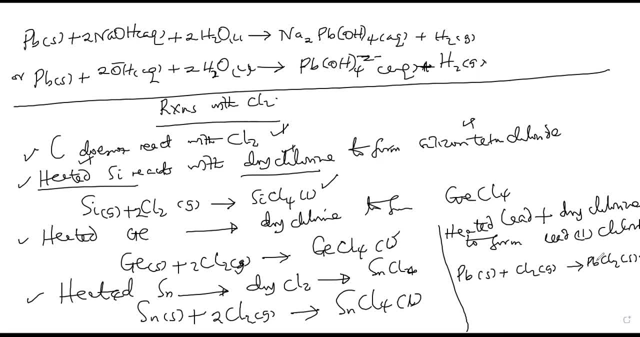 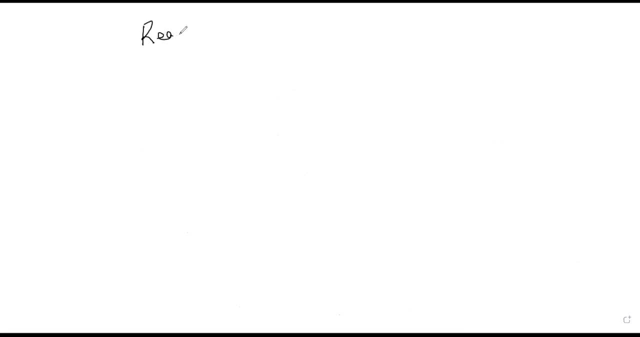 plus oxidation state. We say that for plus oxidation state with lead it is more stable compared to plus oxidation states. Okay, I'm concluding with this reaction, And this is the reaction of group 4 elements, with the sulfur Reactions, with the 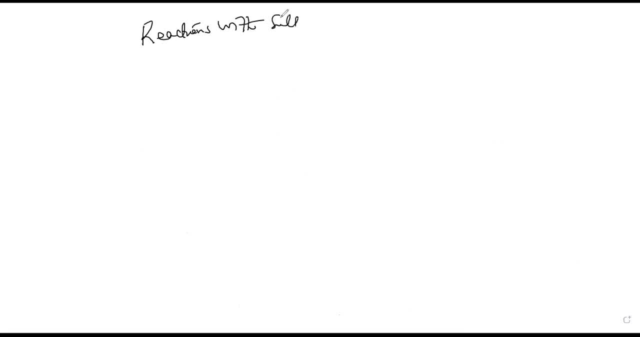 So we have this, So we have this, So we have this. This is what we have, This one. all of them react with sulfur. okay, but they must be heated carbon. we begin with the carbon reacts with the vapor of sulfur, as i call it, sulfur vapor. 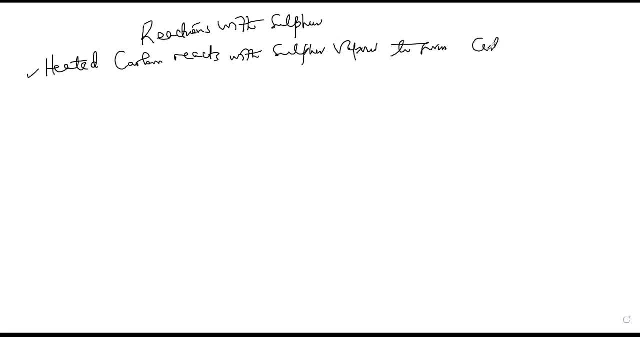 to form carbon disulfide. so you can write the equation carbon plus sulfur vapor. you form carbon disulfide and it is in liquid form. heated silicon reacts with the sulfur vapor to form silica. 4 sulfide form: silicone for sulfide. equation: silicon plus sulfur vapor. 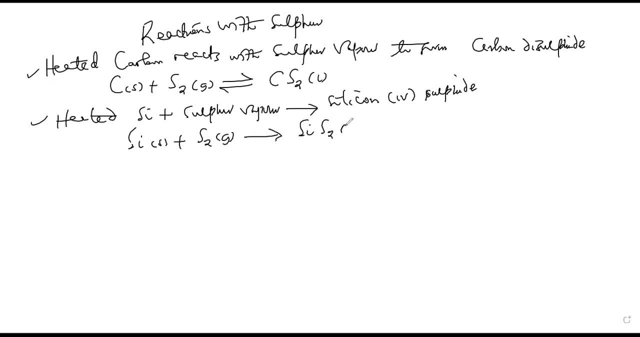 we form siliconified vapor for sulfide. this is a solid. it is only compounded sulfide, that is a liquid. others we form solids. heated germanium works with the sulfur vapor and here we form germanium for sulfide, germanium for sulfide, so you'll have germanium. 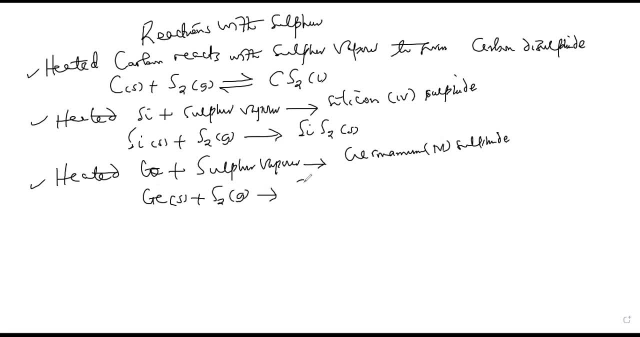 plus surf vapor you form germanium for sulfide. even heated tin reacts with sulfur vapor to form tin to sulfide 14. we form tin to sulfide because as you go down the sulfides that the oxidation state of the plus four decreases, so we shall have a tin.